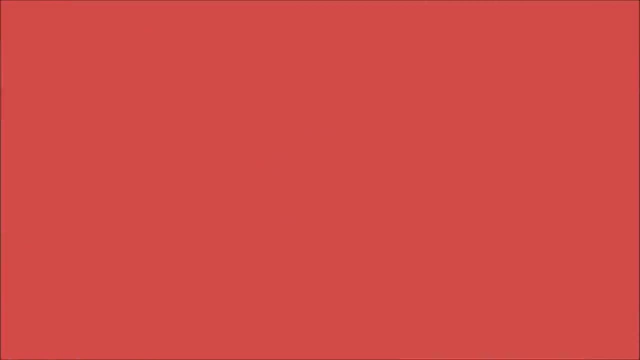 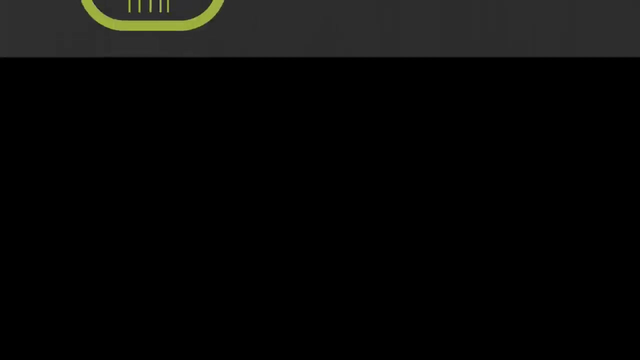 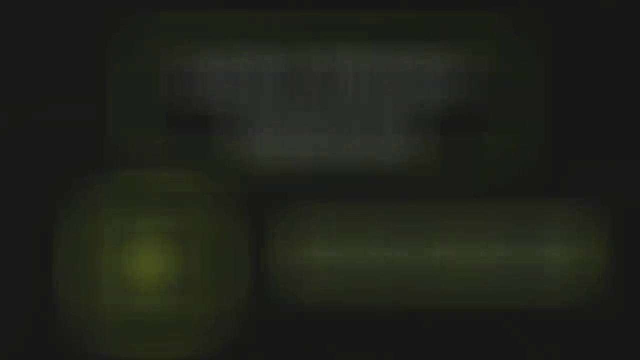 Hey friends, welcome to the YouTube channel. ALL ABOUT ELECTRONICS. So in this video we will understand what is cache memory in computers and the laptops. So in this video we will see what is the importance of this cache memory. What is the typical size of this cache memory? 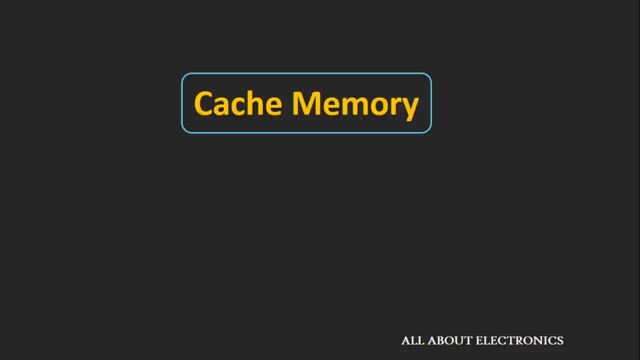 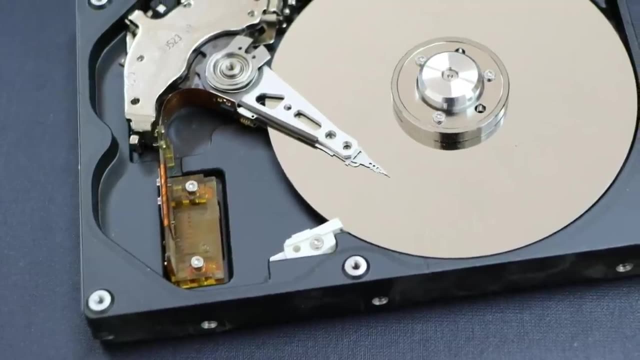 And what are the different levels of cache memory that we find inside the computers. So before we understand this cache memory, let's see different kinds of memory that we see inside our computers. So the first kind of memory that we find inside our computers is the non-volatile kind of. 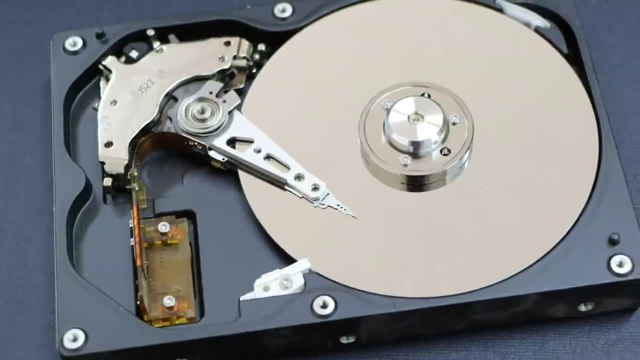 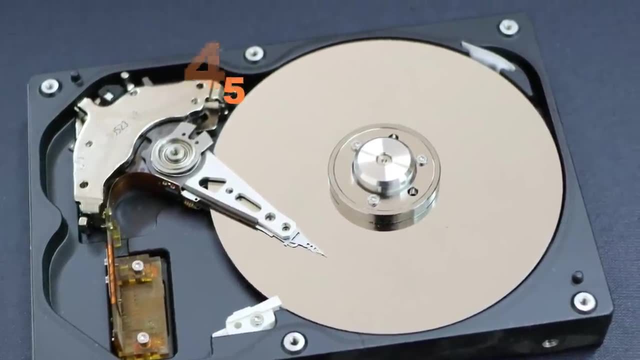 memory like a hard disk drive. So this hard disk drive contains a mechanically rotating fast disk, which is also known as a platter, And if you see any commercially available hard disk drive, the typical rotation speed of this disk is either 5400 or 7200 RPM. 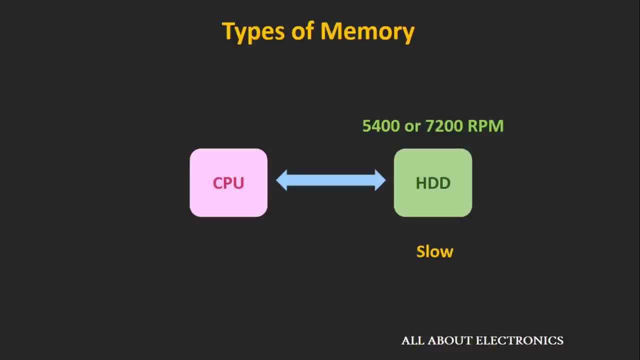 So as this hard disk drive contains a mechanically rotating part, so in terms of the speed they are quite slow. So the typical read or write speed that you get with this hard disk drive is in the range of 80 to 150 MB per second. 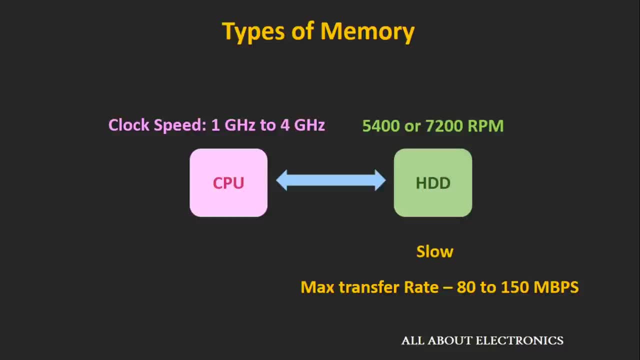 But if you see the clock speed of the CPU, it is in the range of 1 GHz up to 4 GHz. So even though the processor is capable of accepting the data at much higher speed, but it cannot get the data through this hard disk drive at the same rate. 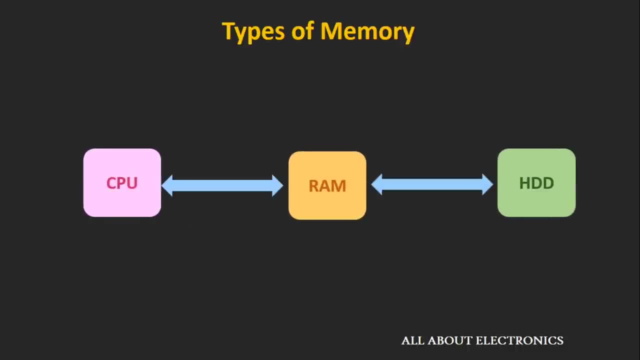 And that is where the second kind of memory comes into the picture, that is, a random access memory. Now, this random access memory is faster compared to the hard disk drive, So this RAM can provide data to the CPU at a much faster rate compared to the hard disk. 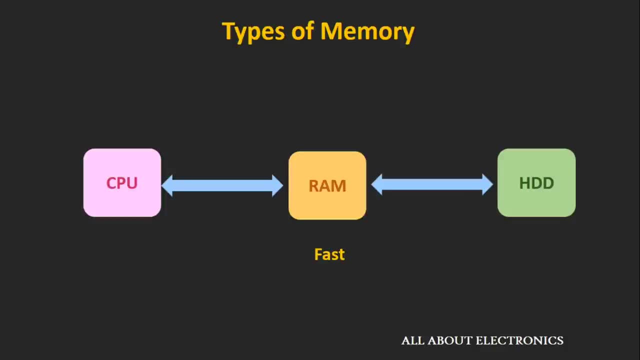 drive, But still it is slower than the clock speed of the CPU. So the typical speed of the RAM is in the range of 400 MHz up to 800 MHz. Still it is lower than the clock speed of the CPU. But if you see the newer generation of the RAMs, like DDR3 and DDR4, then they can operate. 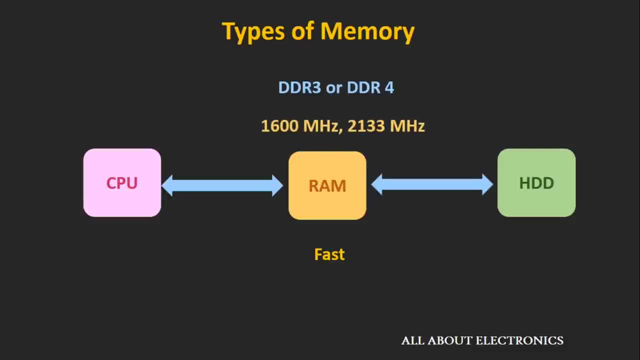 at a much faster rate, like 1600 MHz or up to the 2100 MHz. So now, if you see the speed of these RAMs, they are comparable to the clock speed of the CPU. So now you may say that these newer versions of RAM can supply data to the CPU at the rate 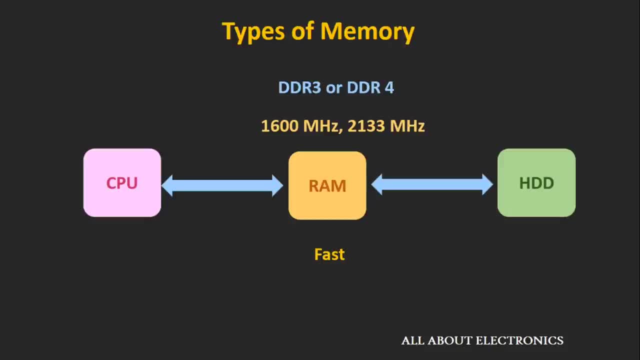 at which they want, But the answer is no. So the modern day processors which we are using are not a single-core processor, but they are multi-core processors. So this processor could be either dual-core, quad-core or maybe even octa-core. 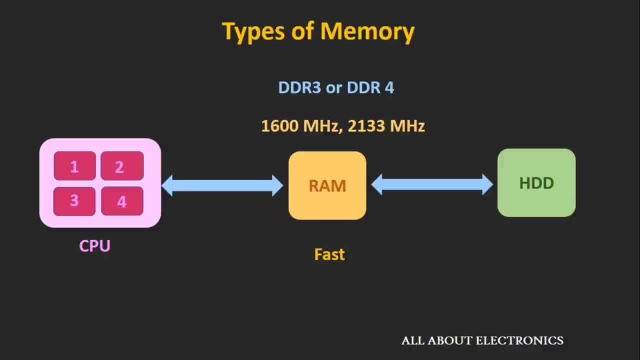 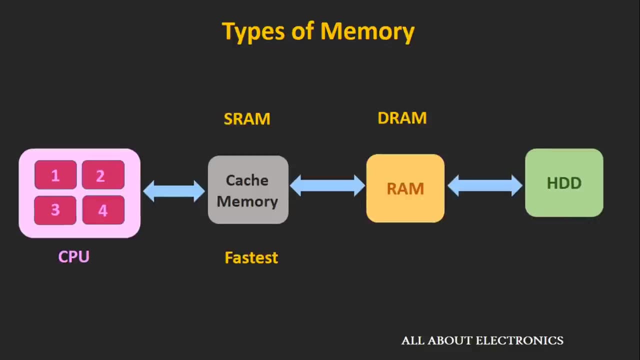 So if all the cores are asking for data at the same time, then this RAM cannot be able to deliver the data to all the cores at the same time, And that is where this cache memory comes into the picture. So this cache memory is fastest among all the memory. 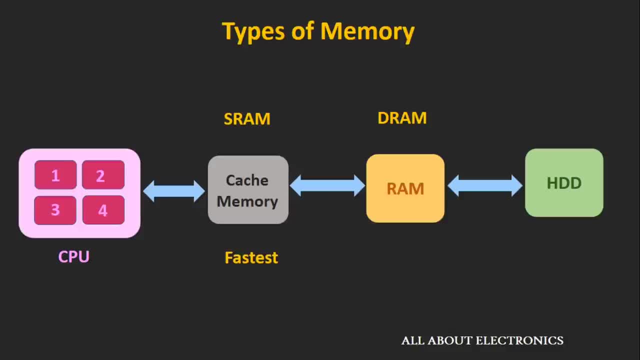 So now, this cache memory is also a random access memory, but it is a special kind of RAM Which is known as a static RAM. So, unlike the dynamic RAM Which we find inside the normal RAMs, this static RAM is quite fast, And the typical size of this cache memory is in the range of kilobytes up to the megabytes. 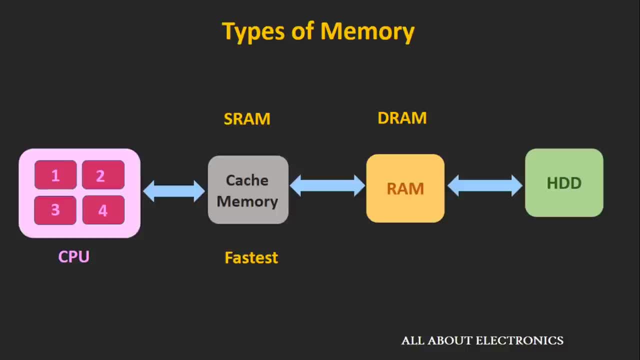 So the data which is frequently required by the CPU can be supplied by this cache memory. So, generally, some instructions and some data which is required by the CPU is stored inside this cache memory. So now let's see the different levels of this cache memory. 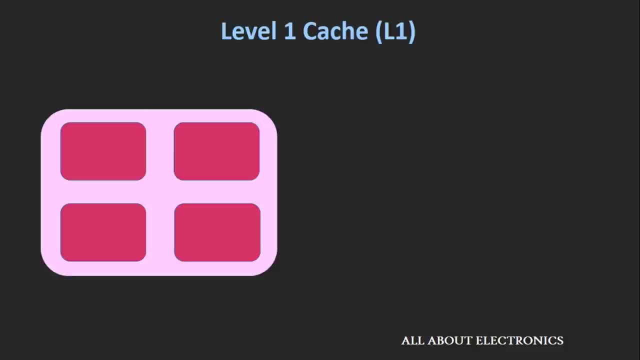 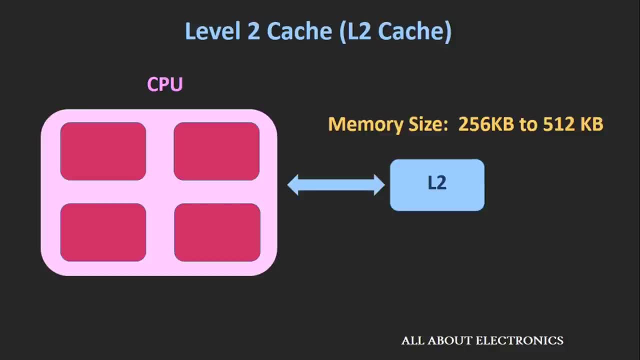 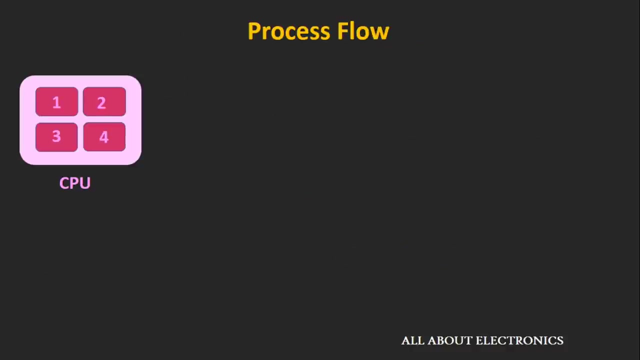 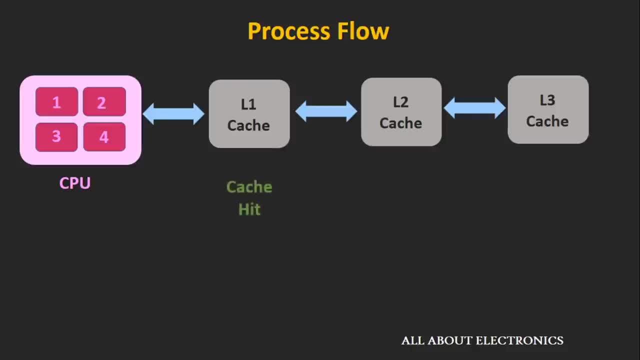 L3 cache. So if the CPU finds the data inside the cache memory then it is known as a cache hit, But if data is not available inside the cache then it is known as a cache miss. So suppose if data is not available inside the L3 cache then the CPU will look inside. 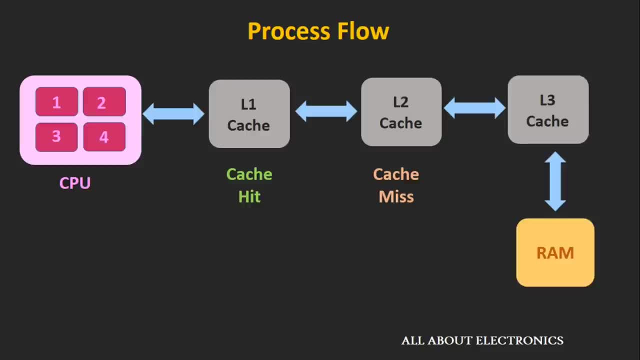 the random access memory or a RAM. And still, if it doesn't find any data inside the RAM, then it will get the data from the hard disk drive. So when you are starting your computer for the first time or you are opening some application, 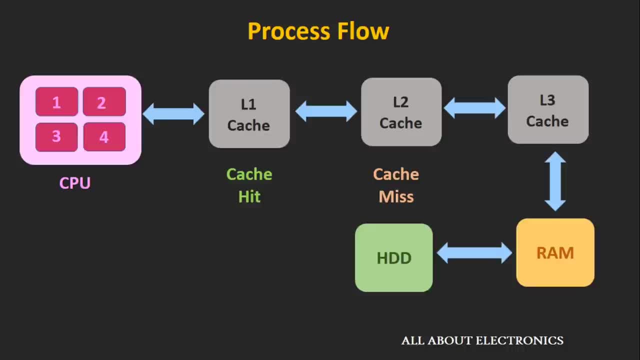 for the first time, then that data will not be available in either cache memory or in the RAM. So at that time the CPU will get the data from the hard disk drive. But once the application is opened and then after, if it requires some data, then CPU will. 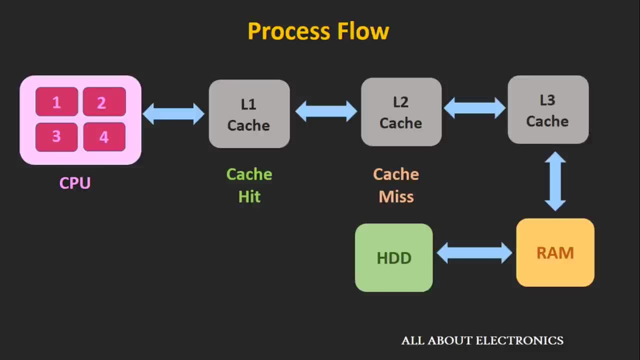 get the data either from RAM or through the cache memory. Now you may ask that if this cache memory is so fast, then why the size of this cache memory is only in the megabytes. So the reason is that this cache memory is much, much costlier than the other memories. 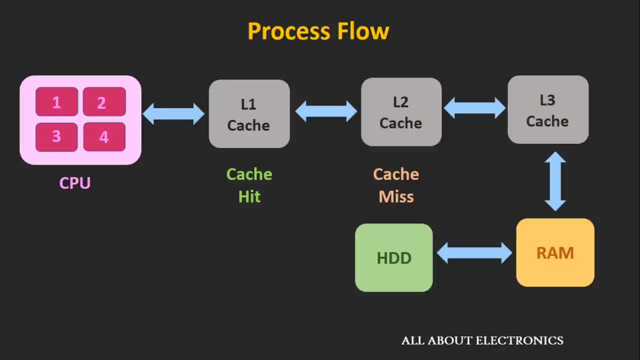 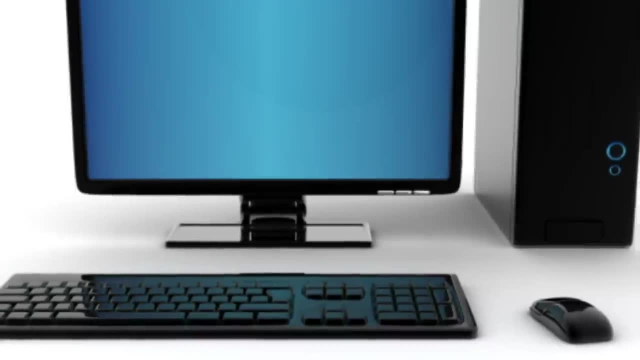 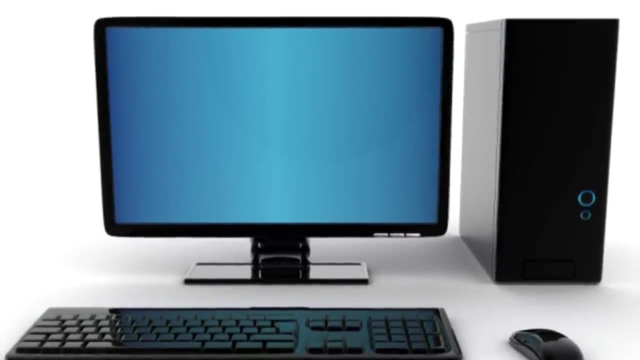 And that is the reason you will find only a few megabytes. So when you are buying some desktop or a laptop for yourself, don't only look the random access memory, but also look the how much cache memory that CPU has, Because this cache memory decides the overall performance of the processor.